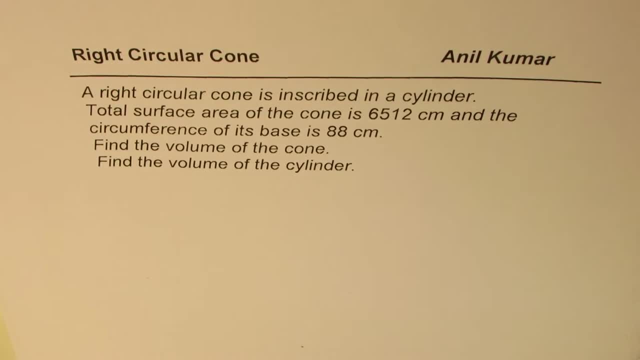 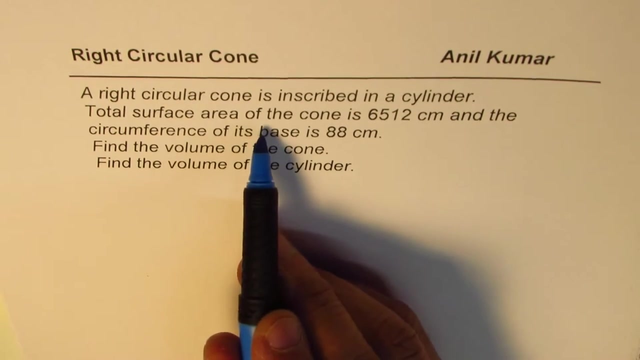 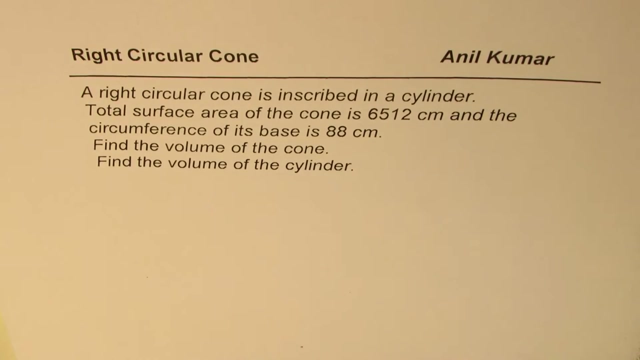 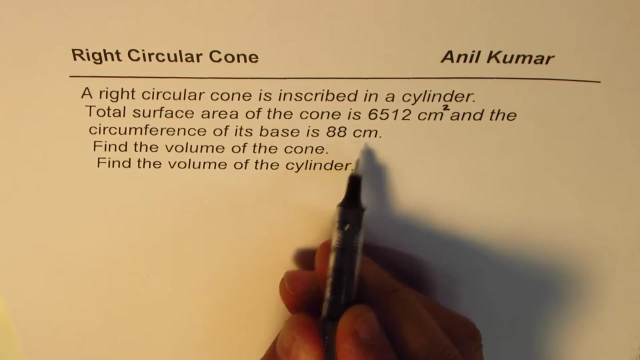 I am Manil Kumar, sharing with you a question which has been shared by my subscriber. So let me first thank my subscriber for actively participating and giving me opportunity to work with such beautiful questions. The question here is: a right circular cone is inscribed in a cylinder. Total surface area of the cone is 6512 cm square. right It should be square And the circumference of its base is 88 cm. Find the volume of the cone and find the volume of the cylinder. So that's the question for you. 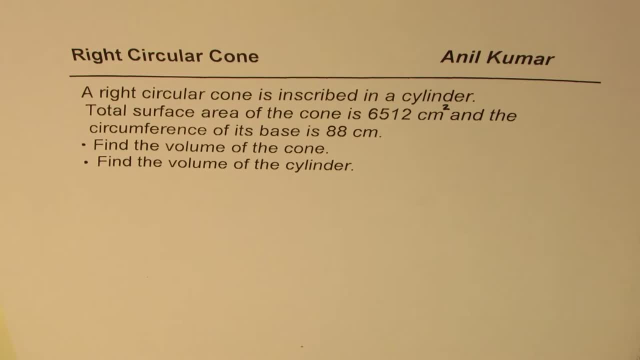 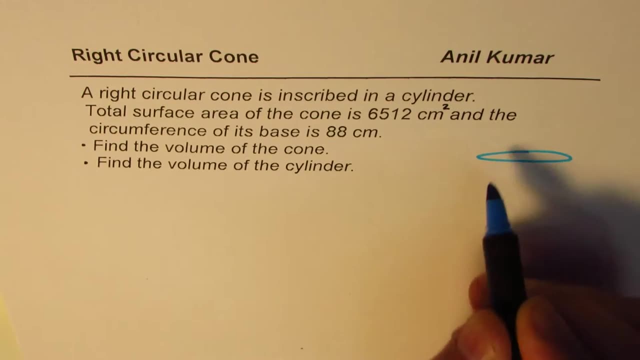 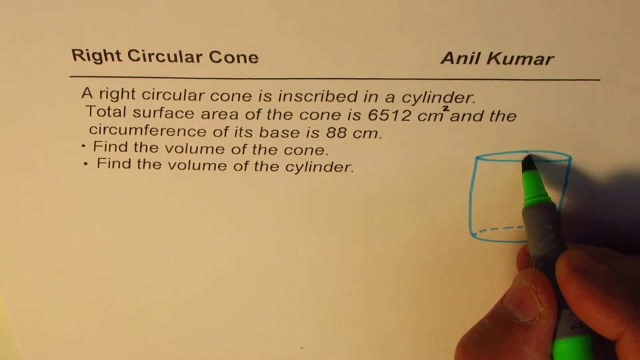 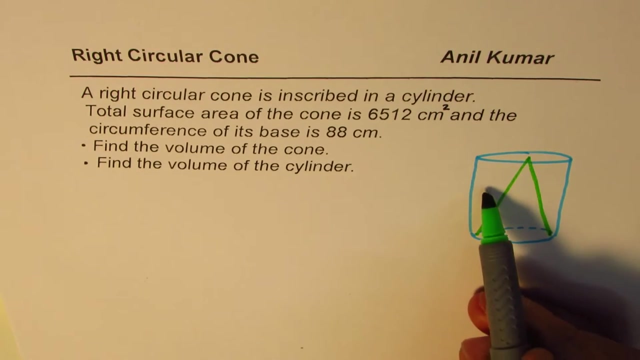 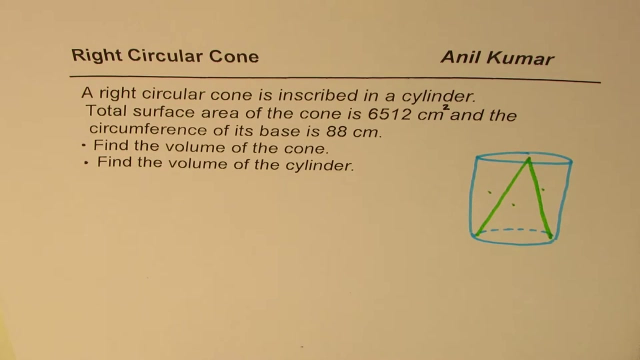 You can pause the video, answer the question And then look into my suggestions. I have three cones in it, right, So that's one thing you should know. So basically, in this question, even if we find volume of cylinder, we can find volume of cone. The multiple is one third, right, So that's important to understand. Okay, let's see how to solve this question. 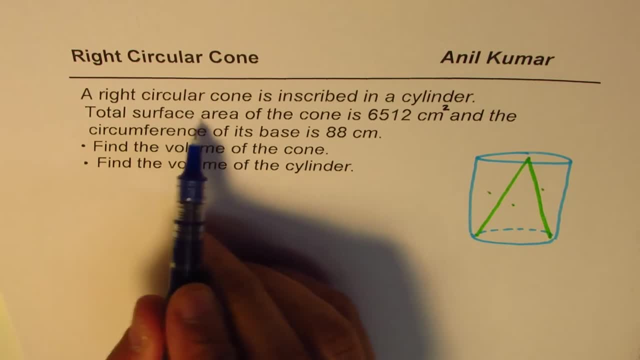 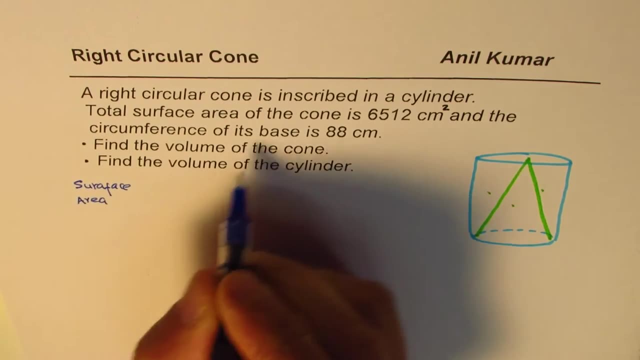 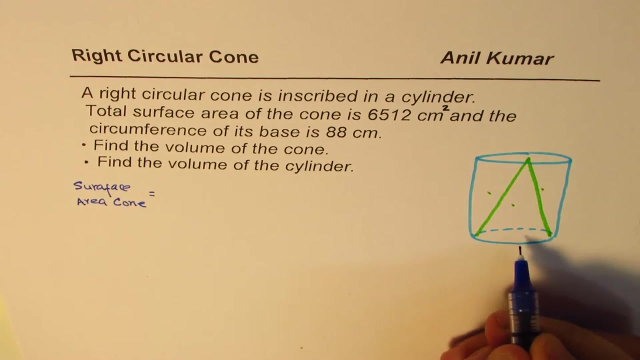 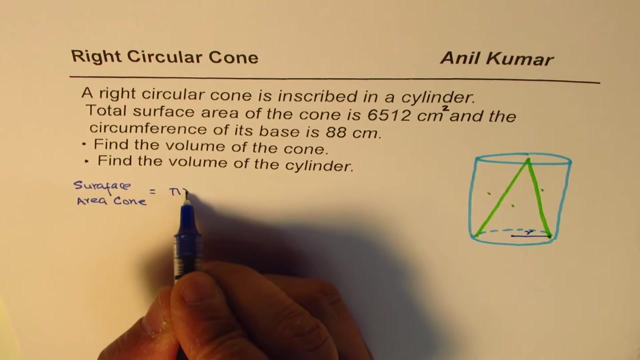 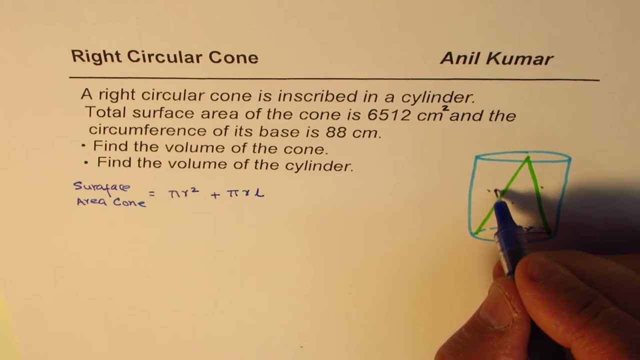 Now, what are we given? We are given that total surface area, right. So we are given surface area of what Of the cone right Of cone. Surface area of the cone is the bottom surface area. If I assume this to be of radius r, then this circle has an area of pi r square right, That's one thing, Plus the lateral area. So this side right, If you open it up, it will give you a rectangle and you can find the area to be as pi r l. where l is this length right? So l is this length for you. 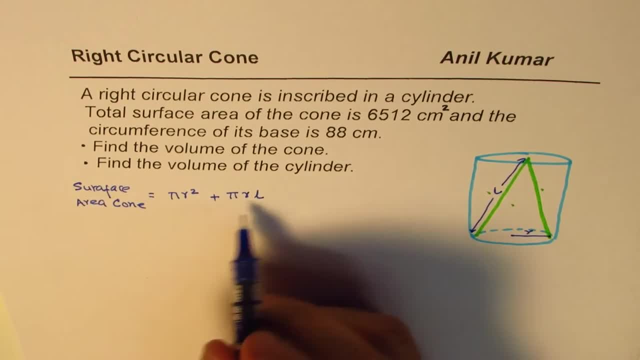 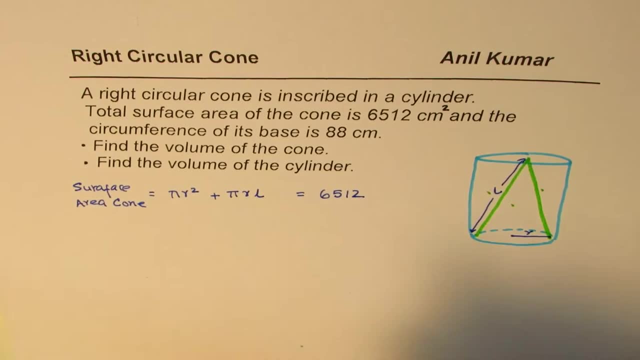 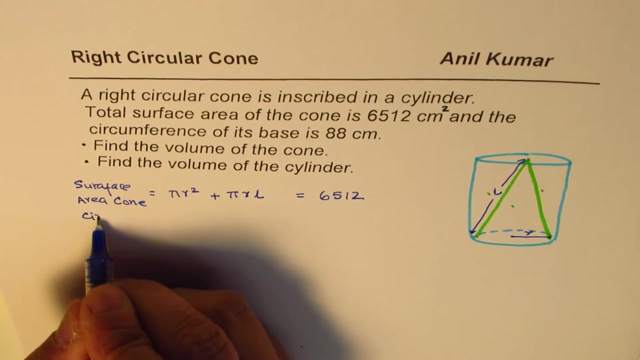 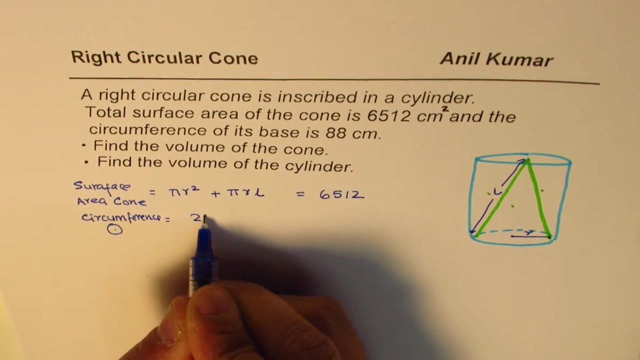 So that's the formula for surface area of the cone. We are given this as equal to 6512, correct, That is what it is. Now we are also given the circumference of the base itself. We know the circumference of the base, So circumference which is of a circle, the formula is 2 pi r right, And that we are given as 88. 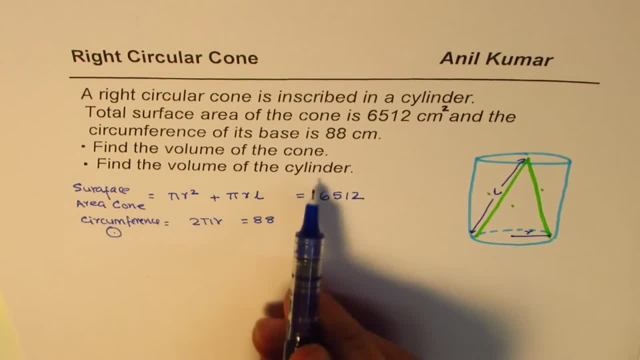 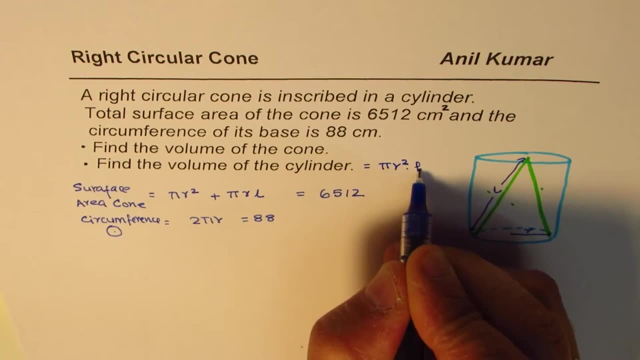 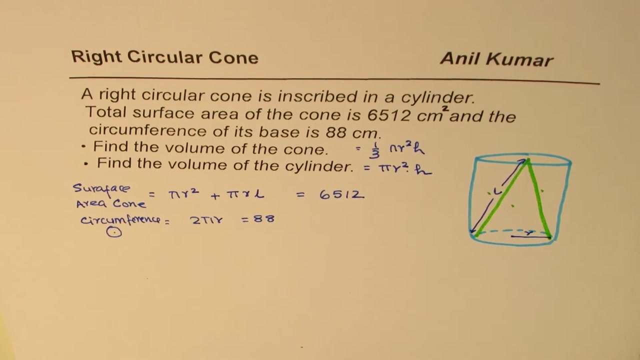 What we need to find is volume of the cylinder. Let me write down the formula here. It is area of the base, which is pi r square times height and volume of the cone. I will write this as one third the volume of cylinder, right? So it is one third of that. So that is how all the formulas are related. Now, actually, you can pause the video, use these formulas and figure out the answer. 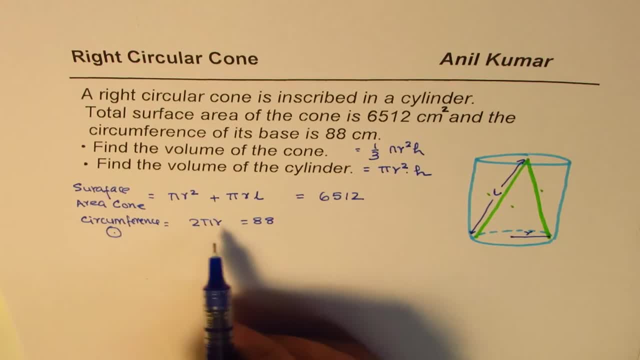 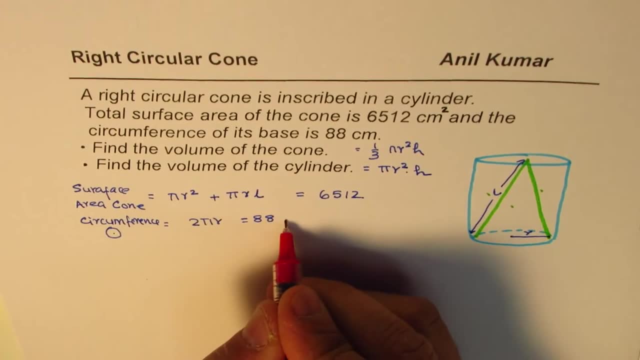 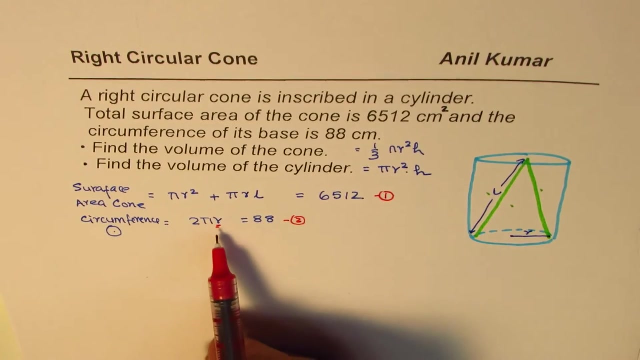 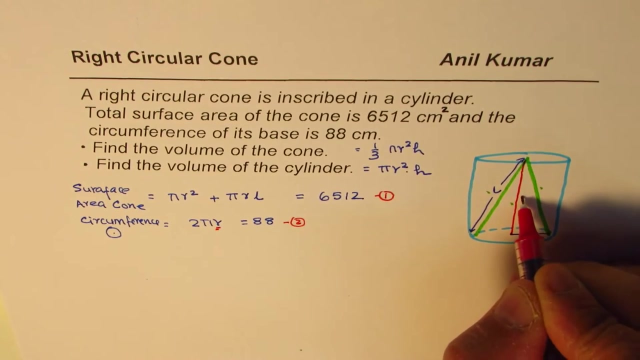 Right, Okay, So our approach here is that from the second equation, which is basically the equation of circumference- this is my second equation and that's my first equation- So from the second equation, let's find r. Once we find r, we can place it there and find l, And after finding length, we can find the height right Using Pythagorean theorem. 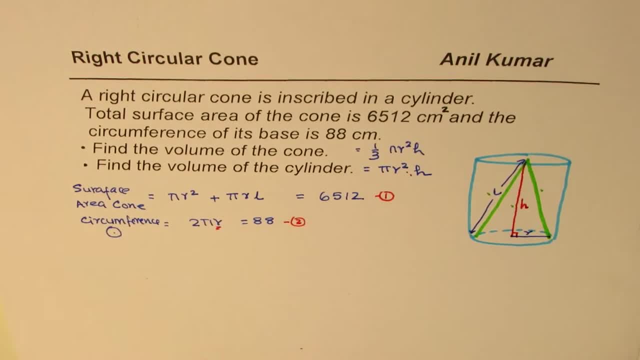 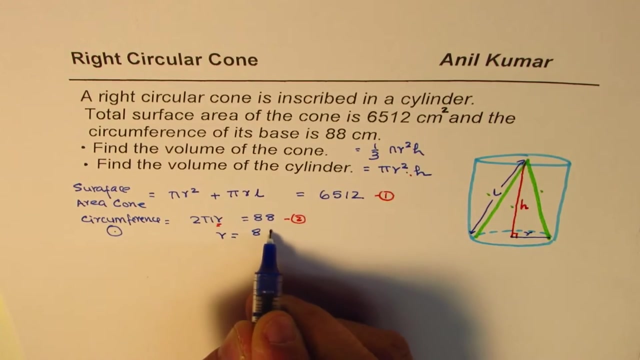 Once we find the height, we can find the volume Right. So these are the steps involved. Perfect, Okay, So let us isolate r and find r from equation 2.. So from here we can say: 2 pi r equals to 88. So r is equals to 88 divided by 2 pi. 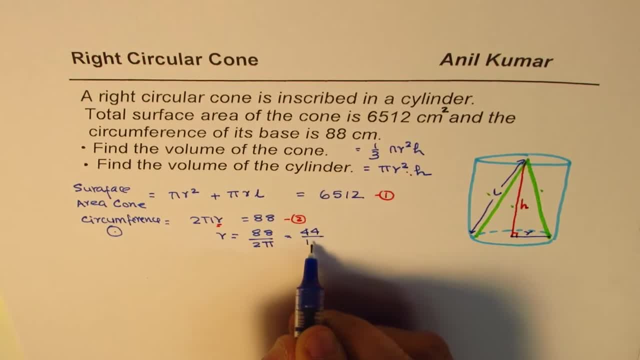 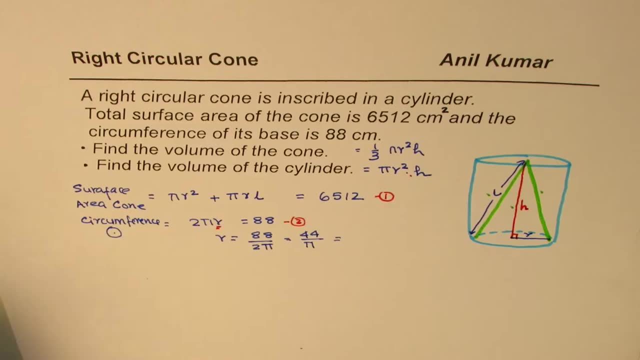 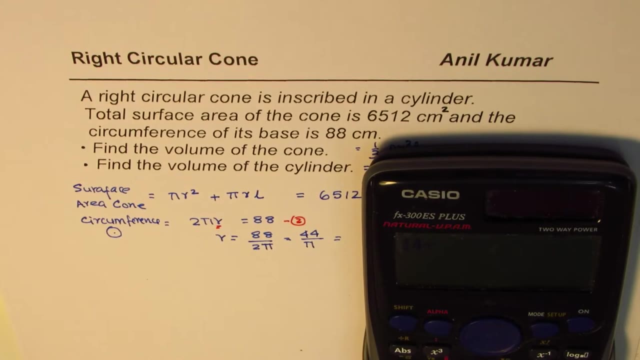 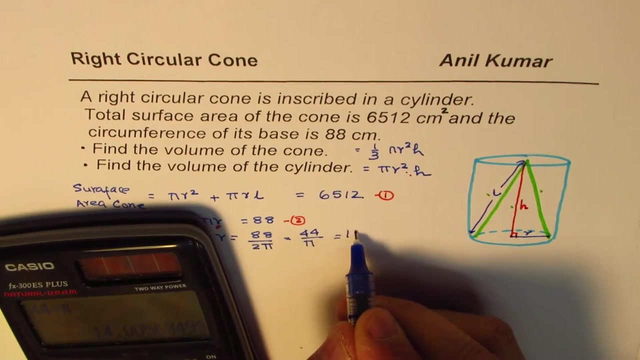 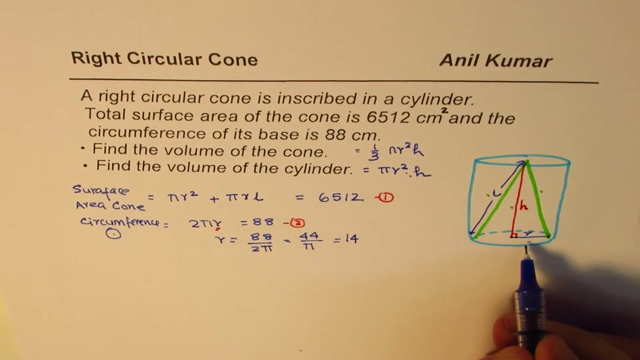 You can keep this as 44 divided by pi, or you could also convert this to decimal numbers, as you wish. Okay, 44 divided by pi. so which is this value equals to 14.0056.. So let me take this value as 14.. Is that okay? So we'll take this value approximately to 14.. Okay, So the radius for us is 14.. Okay, Once we know the radius, let's call this equation as 3.. 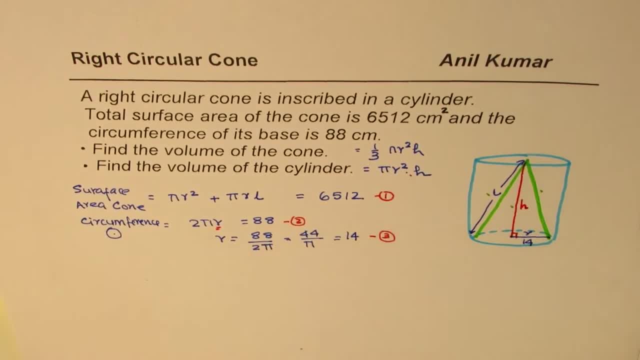 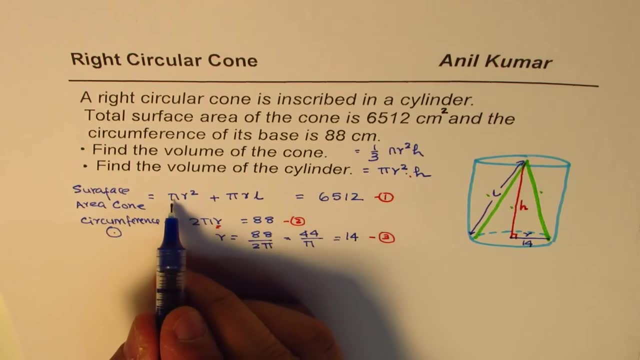 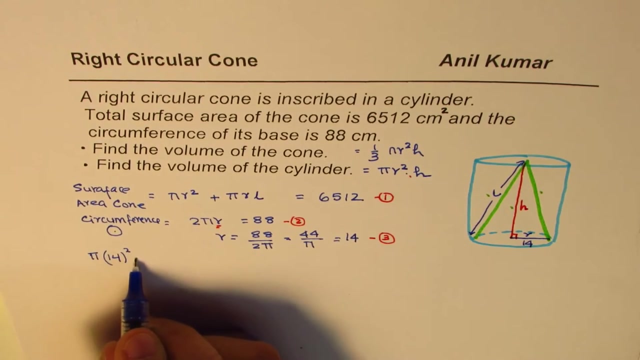 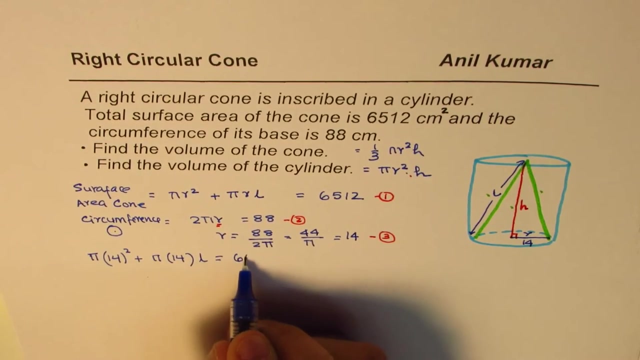 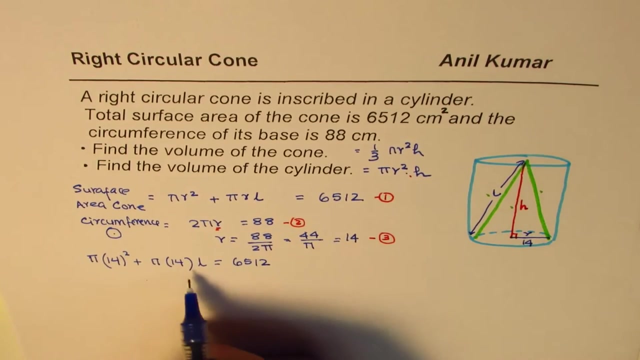 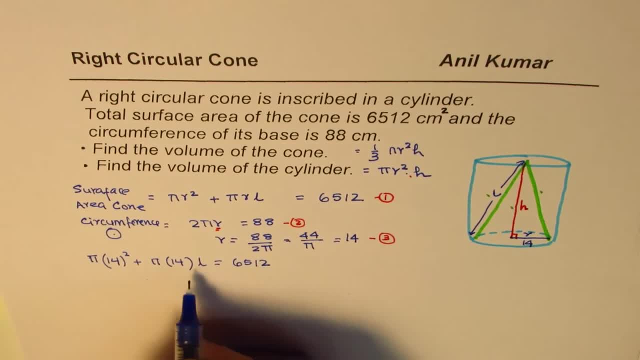 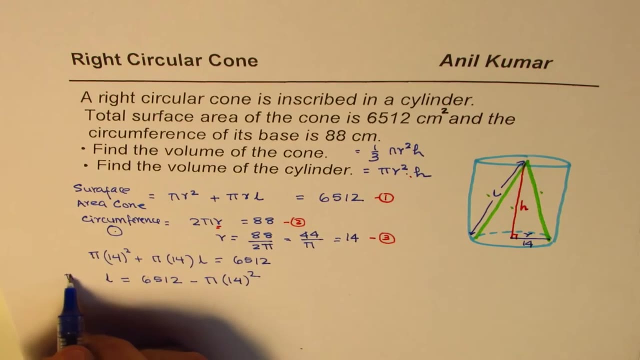 Okay, Okay. So from here we can say: length L is equal to 6512.. So we're going to spices out this xx to become 5, medio 15.. Okay, From perder this, And this is locked in the term, This should be dried out by 8.. 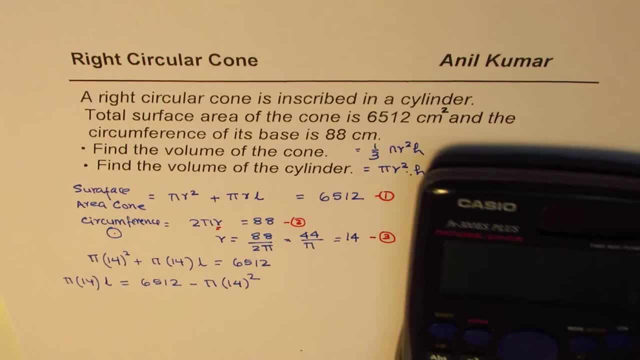 And then y equals this and y equals this. Then you do this 1 by 2.. superficially right, It's of course 5 meters away from is square, square. They detect and find 15 meter away. So we have 6512 to take away. 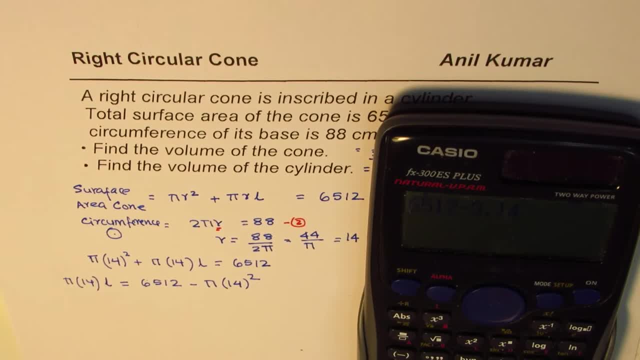 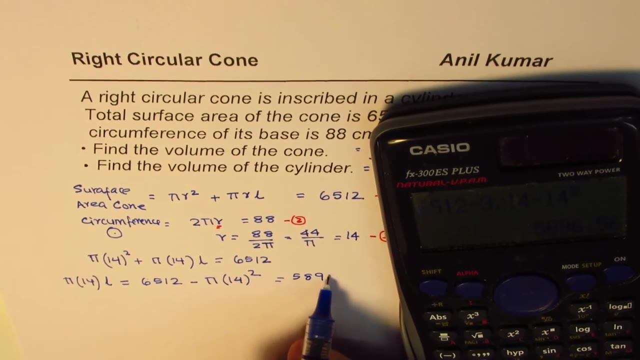 Okay, way, 3.14. this time I am using 3.14, which you can use right times- 14 square, and that gives you- let us round to 2 decimal places: ok, So this is equals to 5896.56. ok, So L is equals. 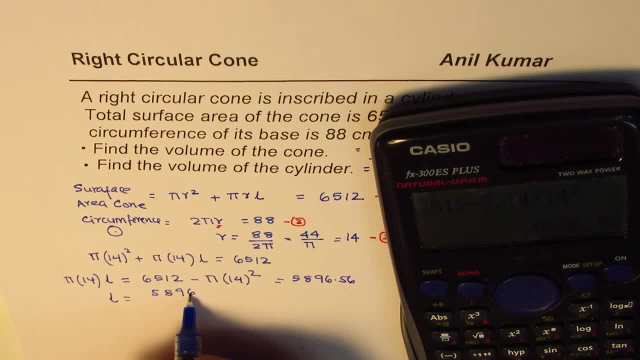 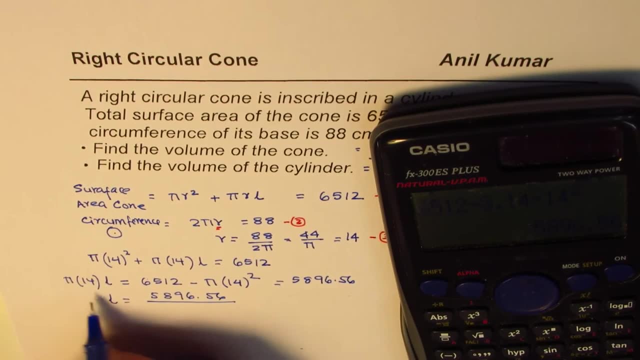 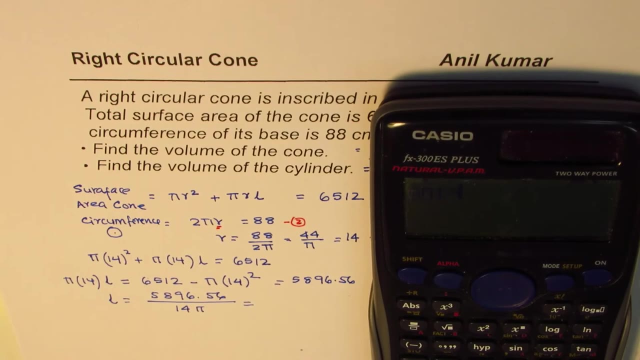 to this number, 5896.56 divided by pi times 14. let me write 14 pi right, So let us do this. So this number we are going to divide by in the bracket, let me write down 14 times pi, which is 3.14. bracket close equal to: So we get a value which is length of 134. 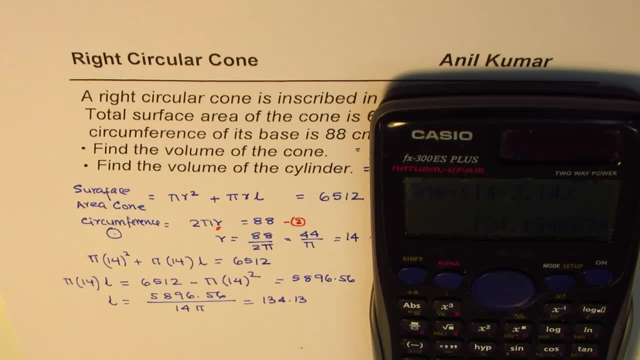 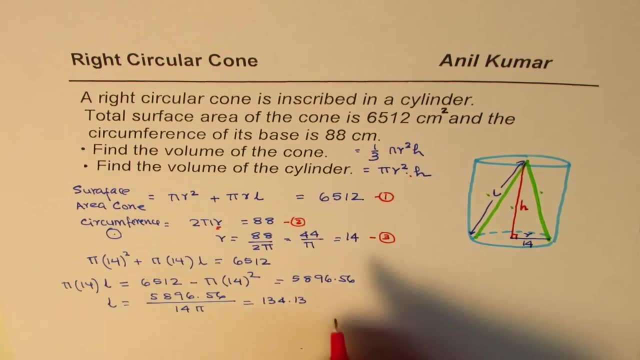 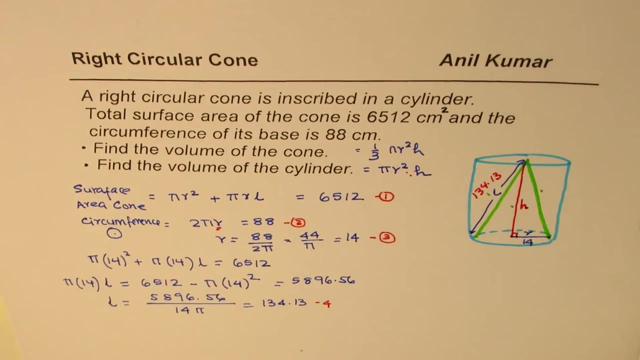 point. let us say 13.. So that is the slant height L. So let us call this as our equation number 4.. So we know L is 134.13. right Now, from here we can find the height h. we can. 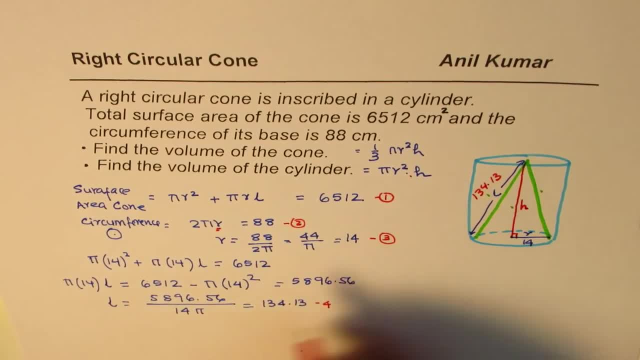 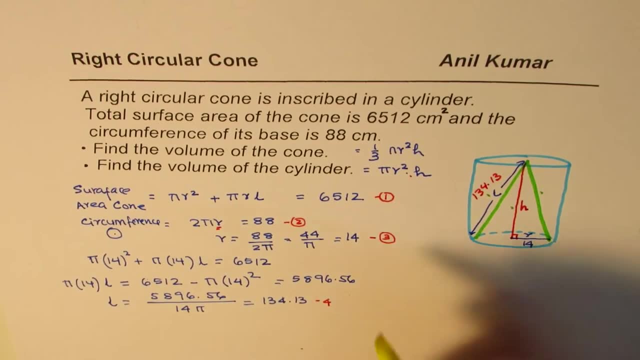 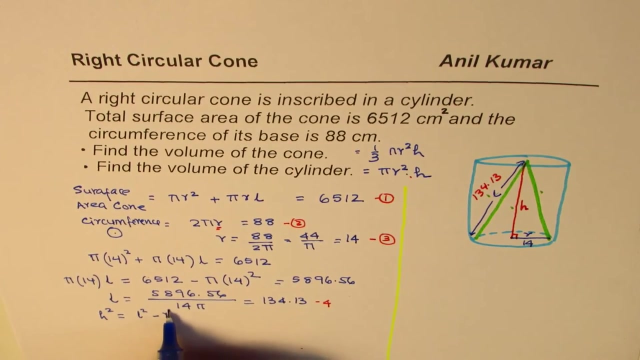 use the Pythagorean theorem to find height. So height squared we can do it here. So h: alright, we are going to find h equal to h. So h here means width, H 5, right, Oh, just to plug out. 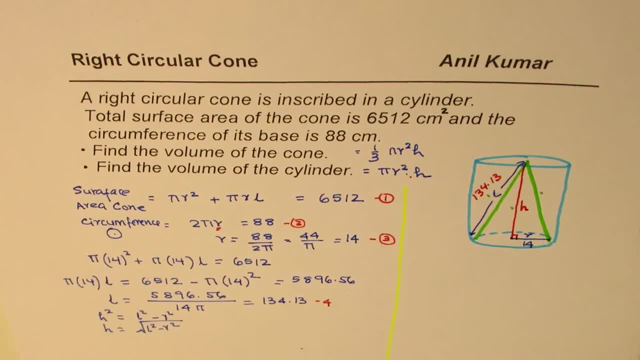 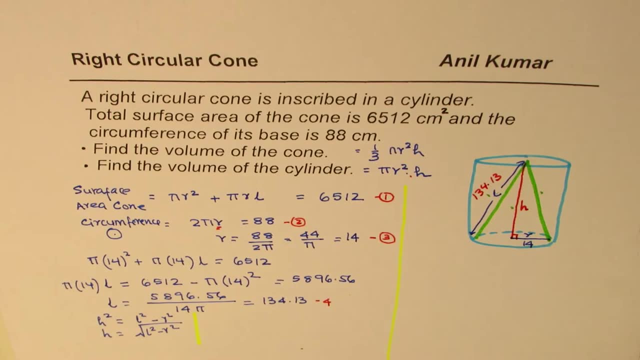 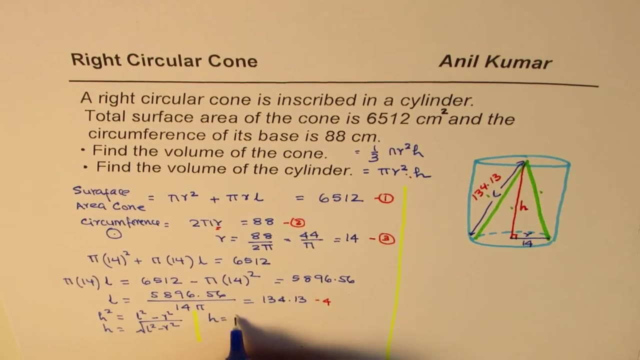 Just to plug out: minus r, square, correct. So that is the formula which we are going to use to find the height of this cylinder or cone, Since they tightly fit, it is inscribed in it. you know the height is common to both right. So we know height is square. root of slant height is 134.13 square. 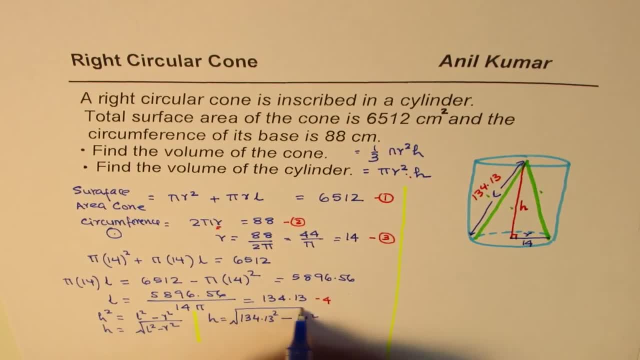 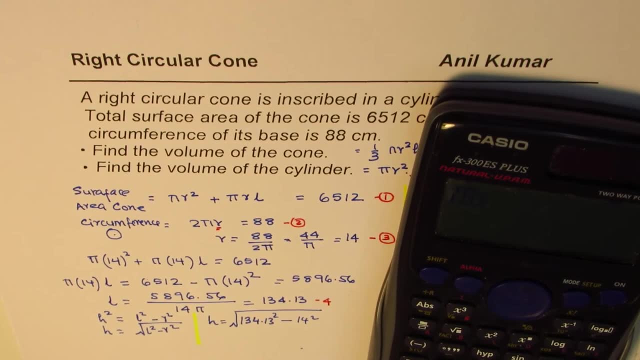 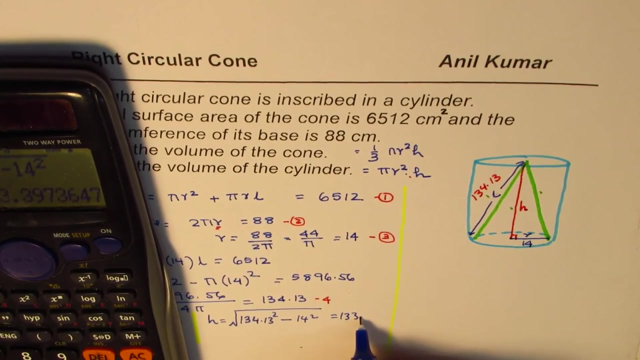 minus radius is 14 square square root. So this is what will give us height. So let us do it. we have within square root 134.13 square. take away 14 square and that is equal to 133.39.. So we get 133.39. let me call this as 133.4, ok. 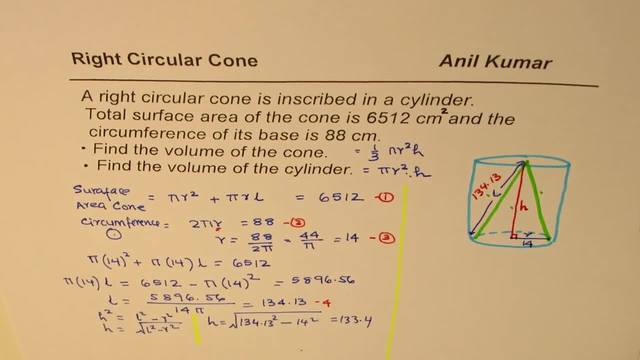 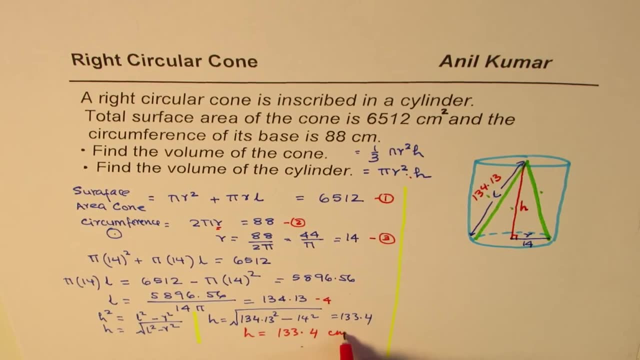 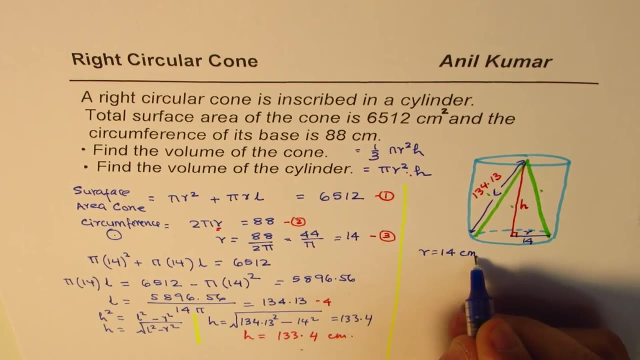 So I am using height of 133.4.. So we have height equals to 133.4. all are in centimeters, correct? So let us write down what all we got. So we have r, which is equals to 14 centimeters height.